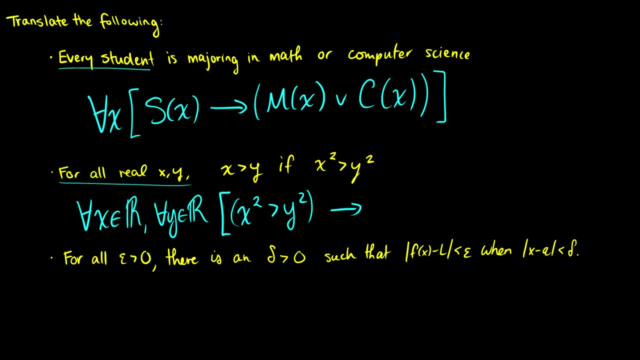 than y. So that's what that one looks like For all x in the real numbers and all y in the real numbers. if x squared is greater than x squared, then x is greater than y. I changed the order of the. if there just a mess with you a little bit, 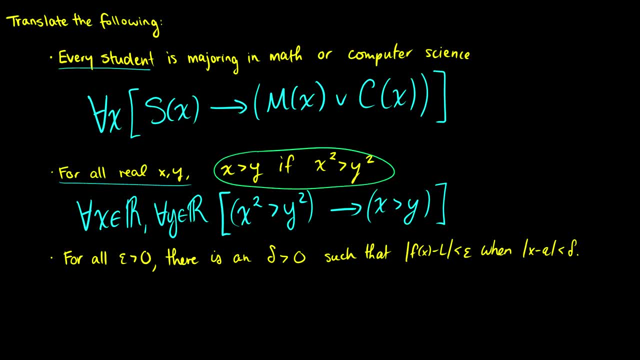 So if x is a data dimension, then y is bigger than y. it okay, the last one for all: epsilon greater than zero. there is a delta greater than zero, such that the absolute value of f of x minus l is less than epsilon when x minus a is less than delta. 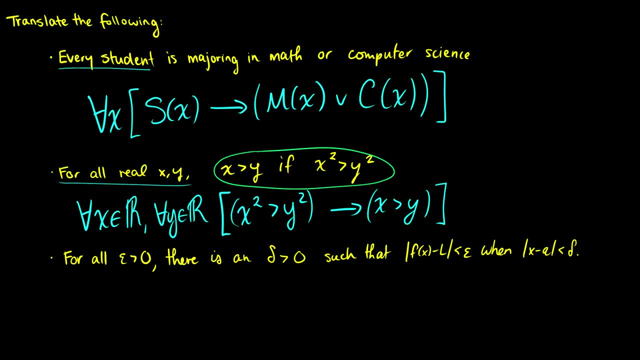 you might see this in a calculus course, so you might be familiar with this. let's change that into quantificational logic. okay, for all epsilon greater than zero, so for all epsilon greater than zero, there exists a delta greater than zero. so there exists delta greater than zero. 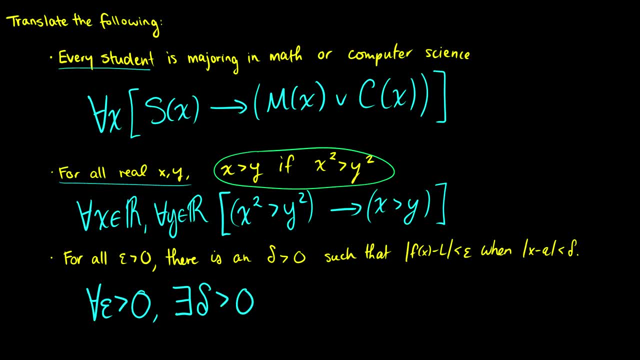 such that- so we can start our bracket here- the absolute value of f of x minus l is less than e when x minus a is less than delta. so this when is just like the if so, when is if so that means that x minus a is less than delta. 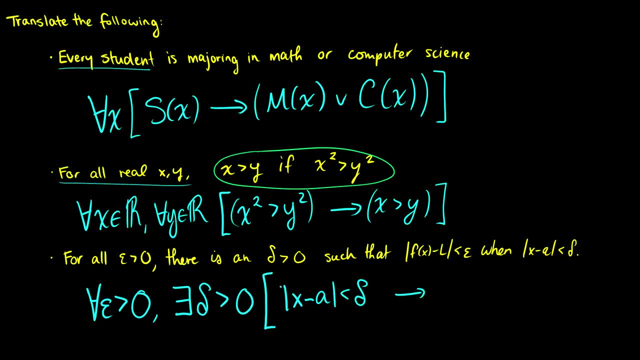 then we get that f of x minus l is less than epsilon. so our translation: for all epsilon greater than zero, there exists a delta greater than zero, such that the absolute value of x minus a is less than delta. then the absolute value of f of x minus l is less than epsilon. okay, so those 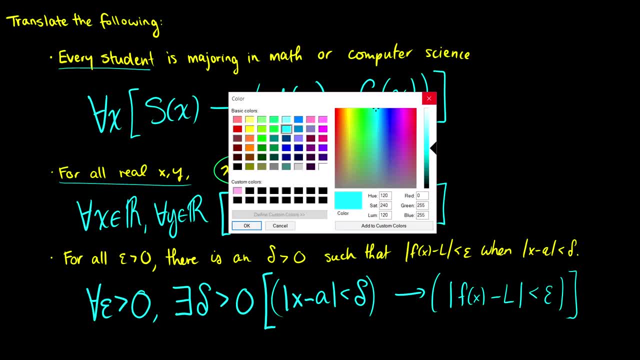 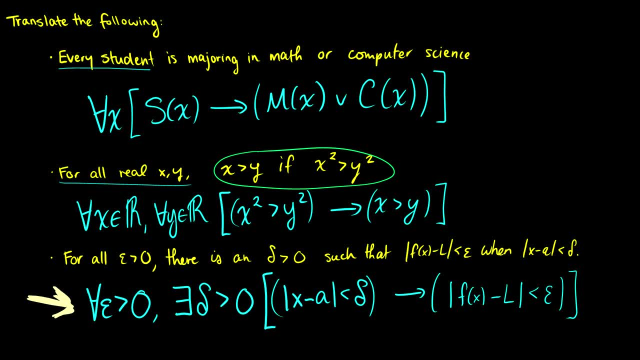 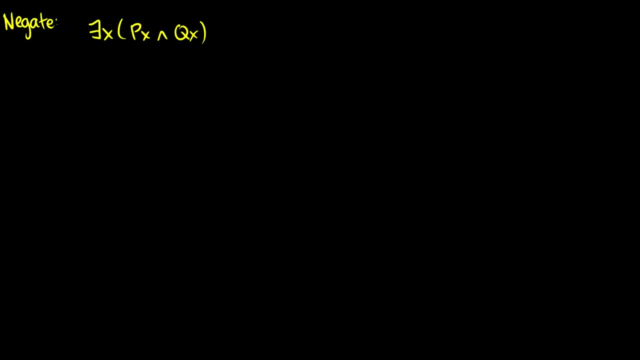 are three translations. i almost guarantee on any. any midterm you're going to get this question. you'll probably get this exact question and you might be asked to negate it. so let's do some practice with negations. negate exists in x, p of x and q of x. so i didn't put the brackets around the p of x and q and x. stylistic choice i. 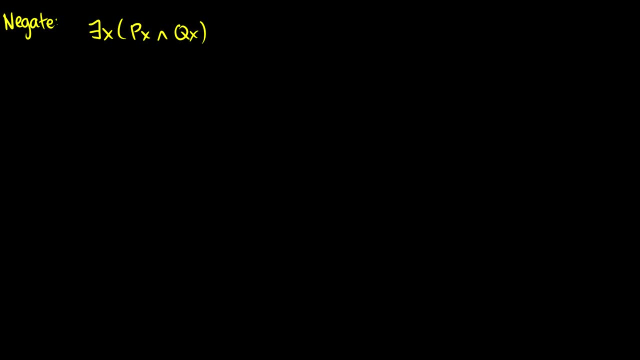 guess. so negate it. so we start negate there exists an x such that px and qx. so first thing we do is we put that negation next to the quantifier. so first step: we want: not exists in x, px and qx. so when we have an encounter like this: not ex or not exists x. 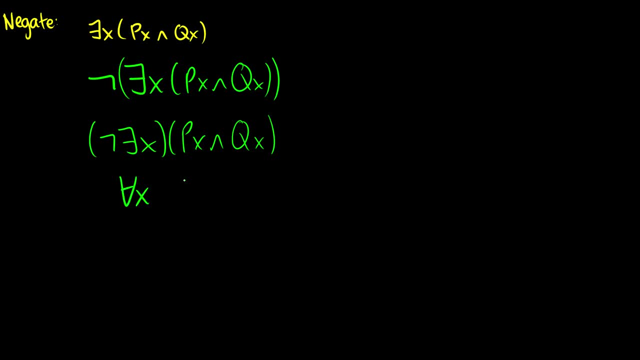 px, we get for all x, not px and qx. so this is how negation works. the negation comes in, it flips the exists to an all and then it negates everything after it. so now we have for all x, and of course we just use de morgan's law here and we get not p of x or q of x. and there you have it. if there does not. 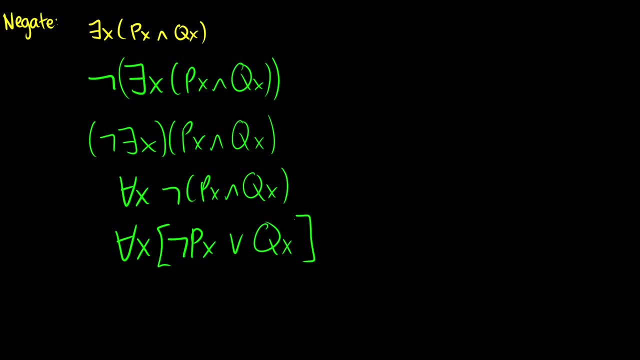 exist an x such that px and qx, then we get not p of x or q of x. and there you have it. that's the same thing. that's saying: oops, there should be a negation here. that's the same thing as saying: for all x, it's either not p of x or not q of x. does that make sense, right? um, i want to say: 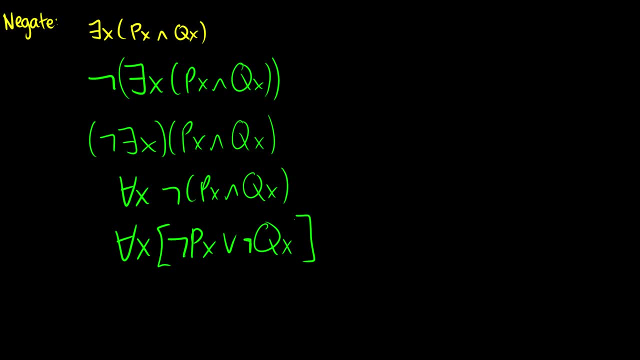 there is some number that is odd or even, okay. so now i'm saying: look, there's no number, that there is not a single number that is odd and even. that's like saying, well, look, all numbers are either not odd or not even. so we have that english translation there that may assist you with this. okay, uh, here's another one. 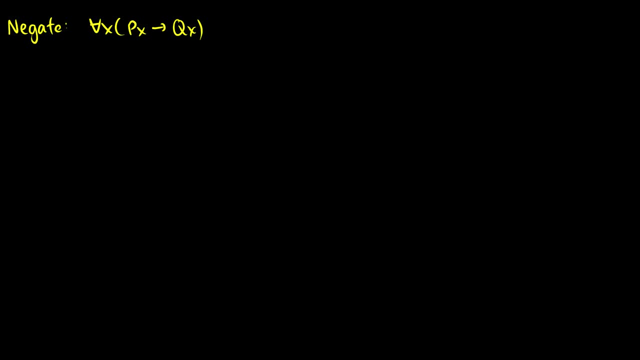 all x px arrow qx. so let's negate this. so we have not all x. again, of course, the screen is being ridiculous here. not all x- px arrow qx. so the first thing, the negation comes in. it flips this all of x to an exists an x and then it negates the rest. so we have not px arrow qx. okay, so we should use the definition. 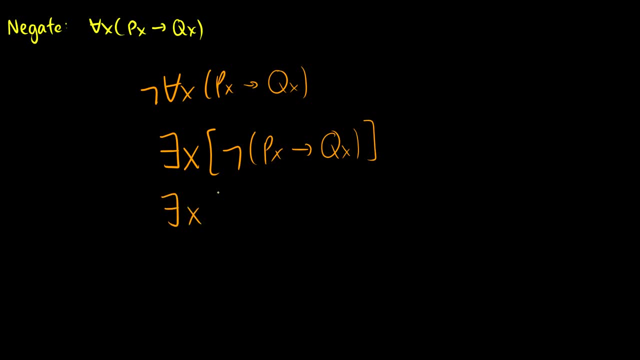 of the conditional here to make this easier to work with. so we have not not p of x or q of x, and then we just used de morgan's law to come in there. so we have not not p of x and not q of x and a.